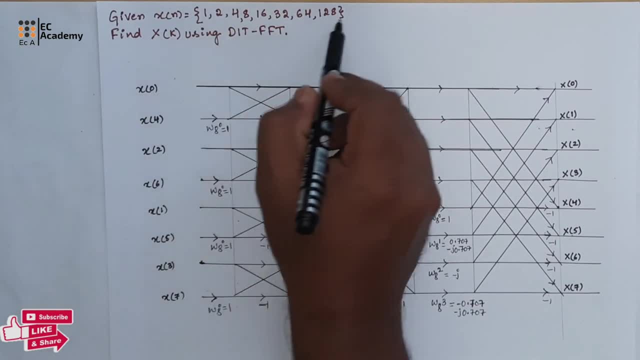 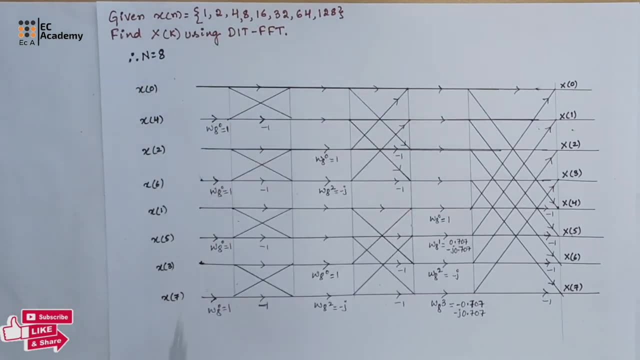 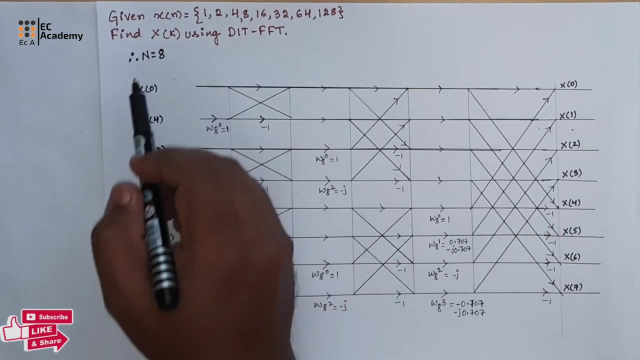 to find x of k. Here. the number of samples in x of n is 8.. Therefore we can take n is equal to 8.. Before doing any calculations you need to draw the butterfly diagram or signal flow diagram, for n is equal to 8.. So this is the standard signal flow diagram for. 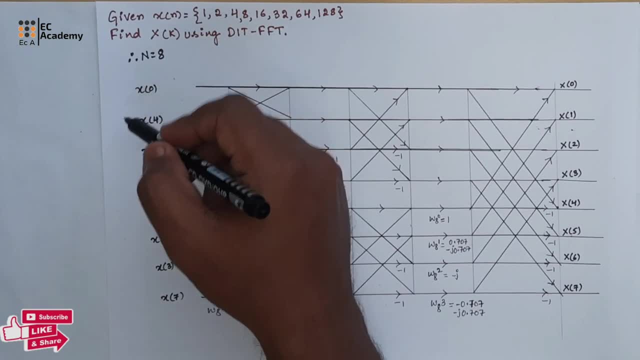 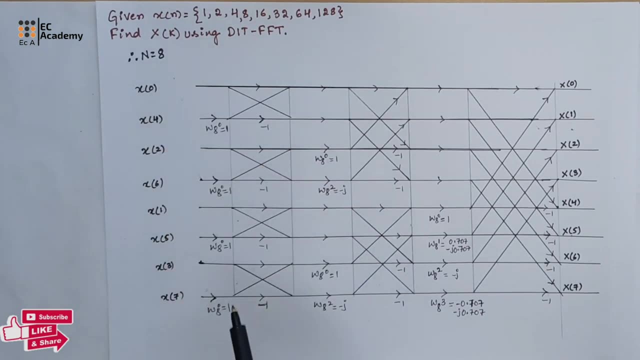 n is equal to 8.. Here the order of time domain signal is decimated. So that is why it is known as decimation, So decimation in time. So here we have written the input as x of 0,, x of 4,, x of 2,, x of 6,. 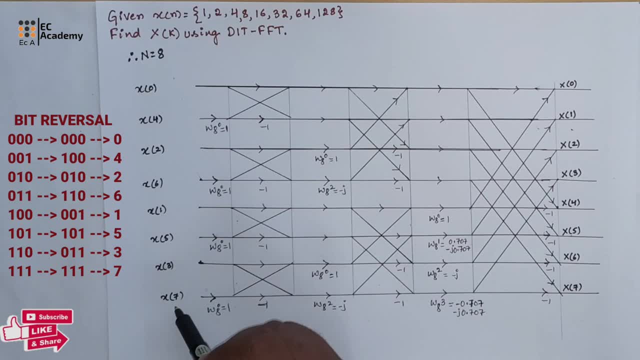 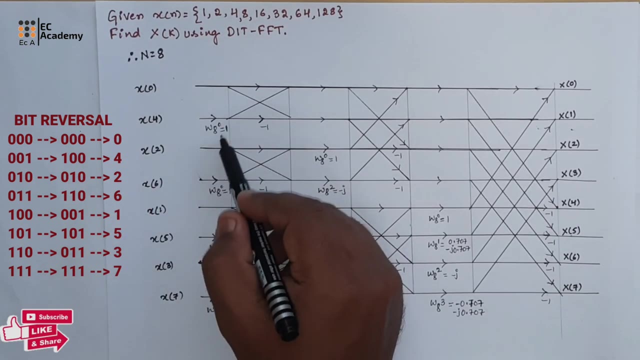 x of 1, x of 5, x of 3 and x of 7.. So this order you can remember, or you can use the process of bit reversal, which we understood in our previous lecture, to write these values. So at the first stage we are having w8 to the power of 0 here. So for that we have 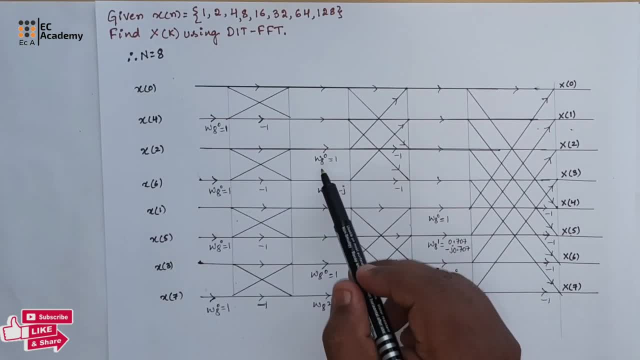 written the value as 1.. And at the second stage we are having w8 to the power of 0 and w8 to the power of 2.. The value of w8 to the power of 0 is 1.. The value of w8 to the power of 2 is minus j. So we 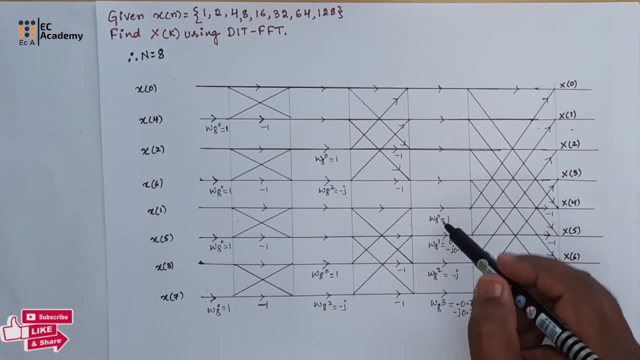 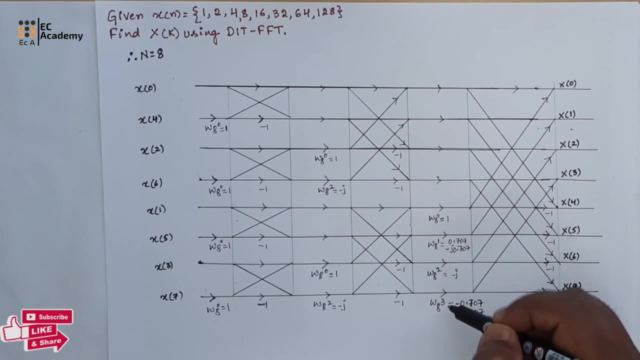 have written the same values here. So in the third stage we are having the value as w8 to the power of 0, w8 to the power of 1, w8 to the power of 2 and w8 to the power of 3.. The values are 1, 0.707 minus j 0.707,. 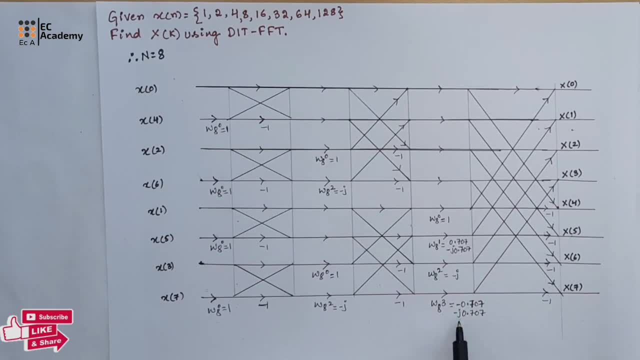 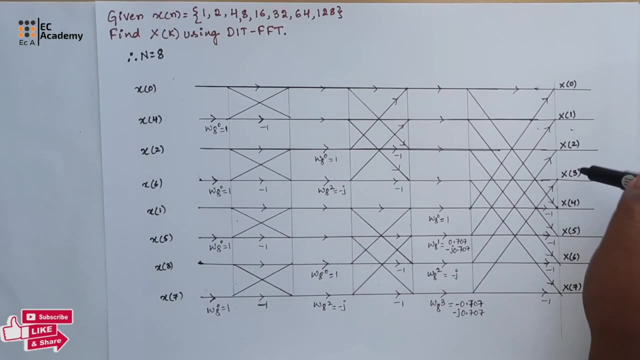 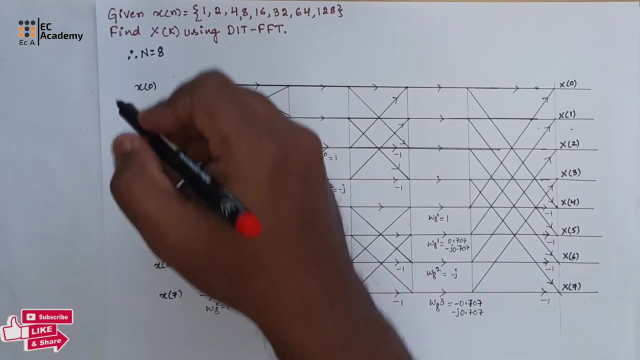 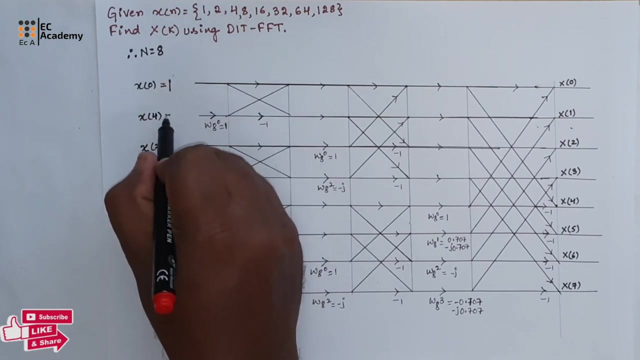 minus j, 0.707.. At the output we are getting the frequency domain signal from x of 0 to x of 7.. In the first step, first let us write the values of all the inputs: x of 0 is 1,, x of 4 is 16.. So from this sequence we can write these: 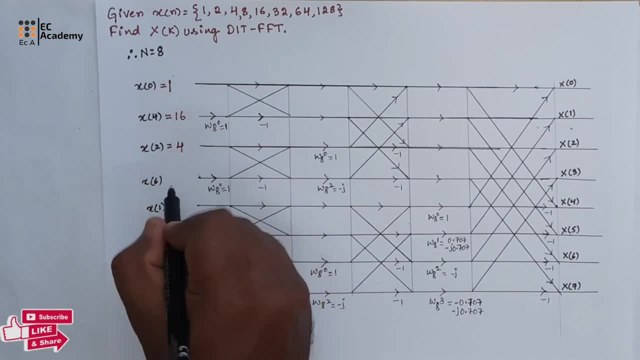 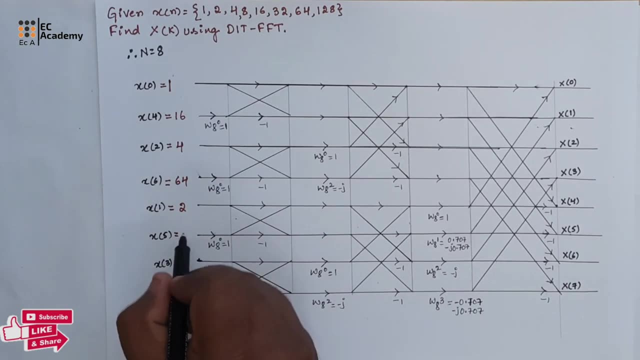 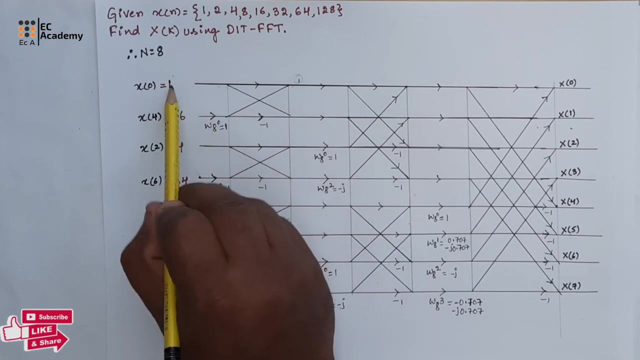 values: 4, x of 6 is 64, x of 1 is 2, x of 5 is 32, x of 3 is 8, x of 7 is 128.. In the first step, we need to find the output here. To find the output at this point, we. 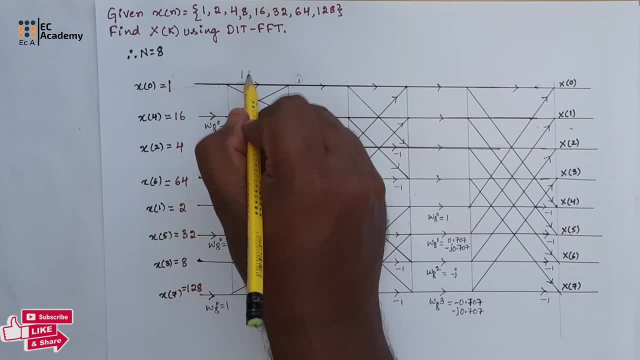 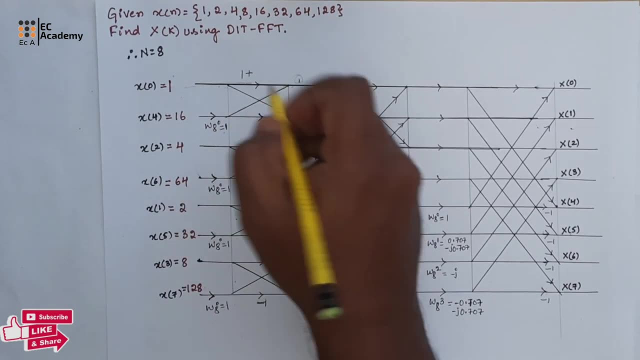 need to take this input here. So let us take 1, we need to add that input with this input on this line. So it is 16 into 1, it is 16.. So it will be 16 here. So the output will. 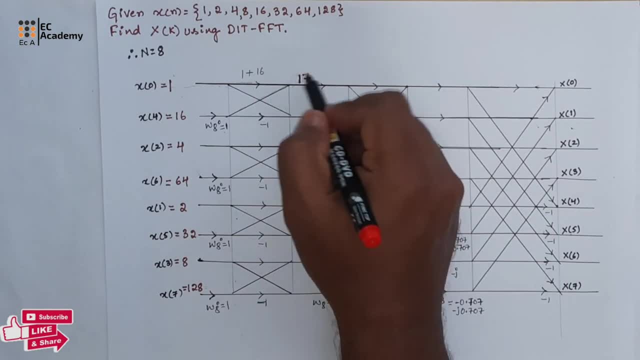 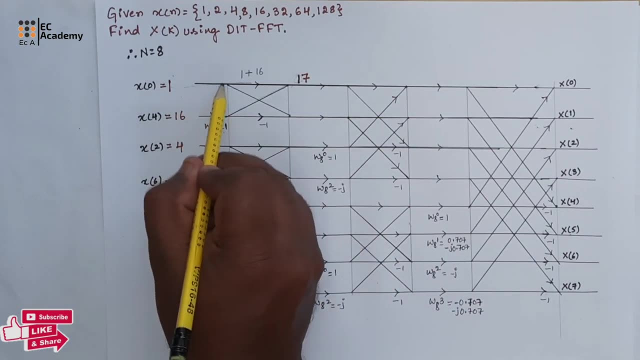 be 17 at this point. So these are the intermediate results that we will get. So to get the output at this point, we should take this input signal, 1 plus so 16 multiplied with 1, it is 16.. Again, it is multiplied with minus 1, so it will be minus 16.. 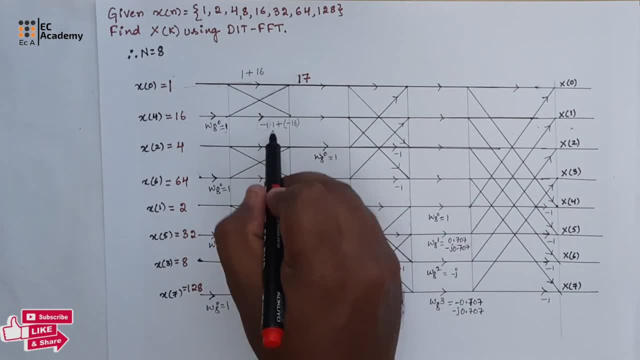 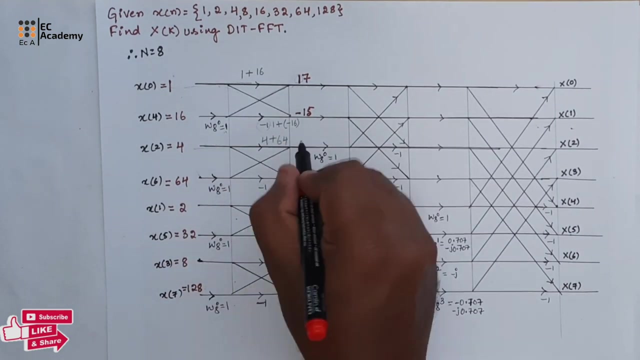 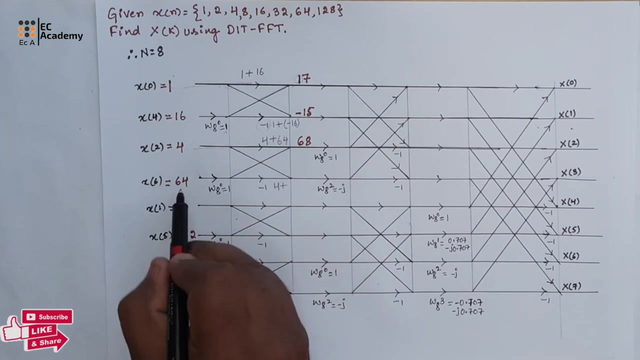 So plus 1 minus 16, it will be minus 15.. In the same way, 4 plus 64, it will be 68.. Output at this point it is 4 plus 64 into 1, it is 64 minus 1, it will be minus 64.. So this: 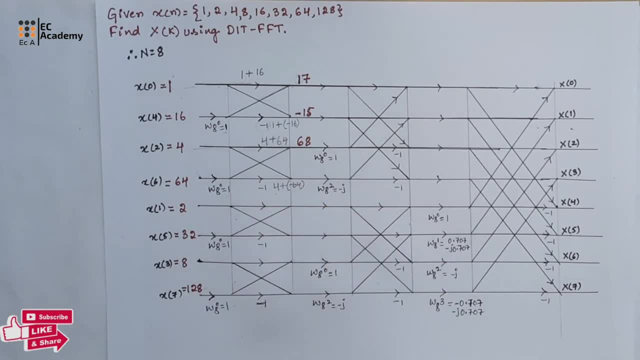 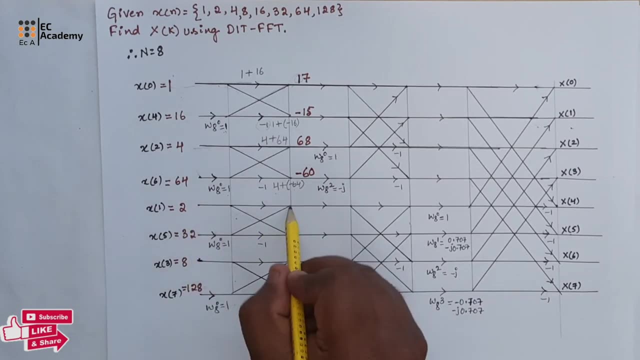 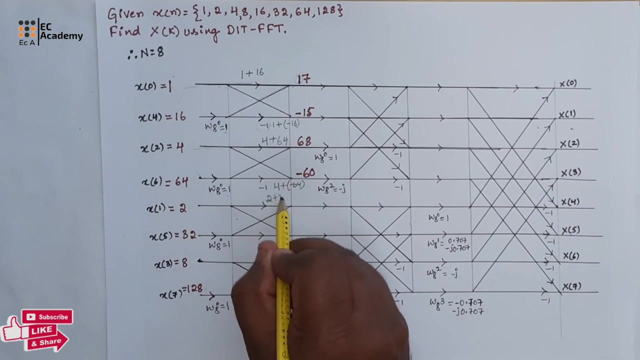 is 64 minus 64 plus 4, it is minus 60.. Again, we need to find output at this point. It is 2 plus 32, it is 34.. We need to find output at this point, which is 2 plus 34 into 1,. it. 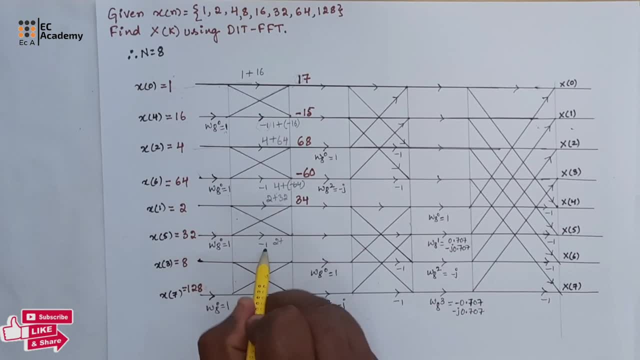 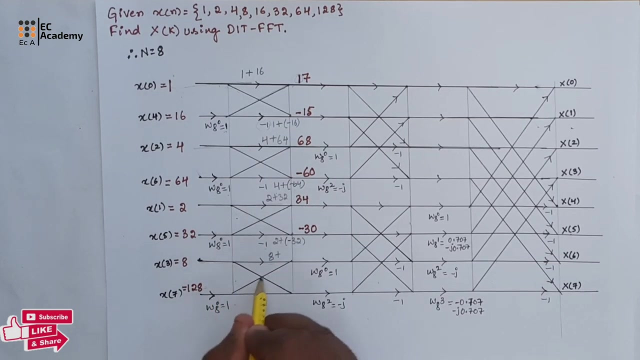 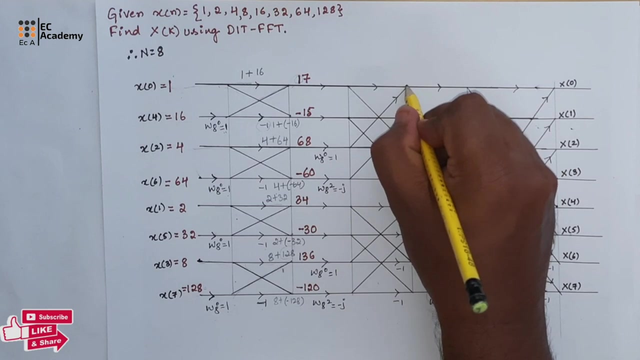 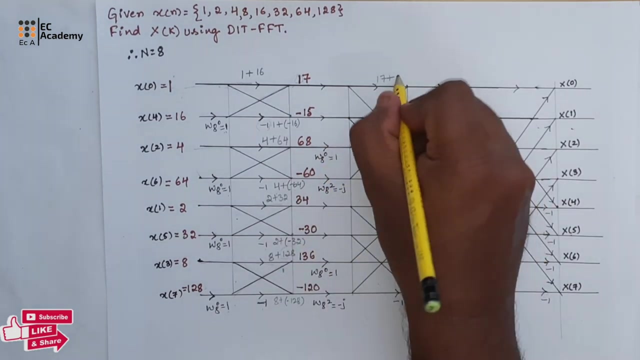 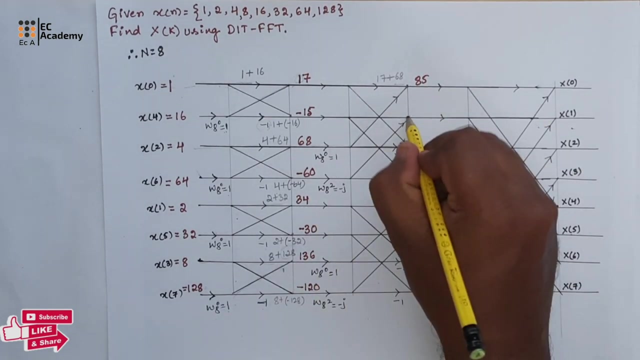 is 34. So that will be 85. Now the output: at this point it is minus 15, so which is on this line? So the line that is joining this point is this one. So you need to trace this. So. 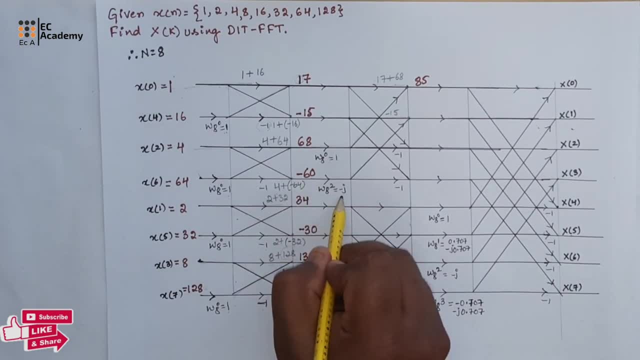 it is minus 60 into minus j, it is 60 j, So it will be plus 60 j. So the output at this point it will be minus 15 plus 64 into 1, it is 64 minus 1,. it is 64 minus 1, it is: 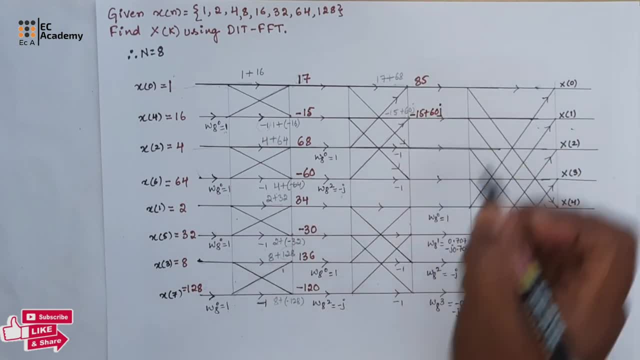 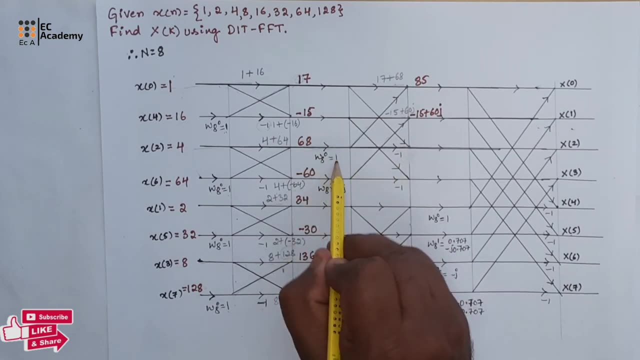 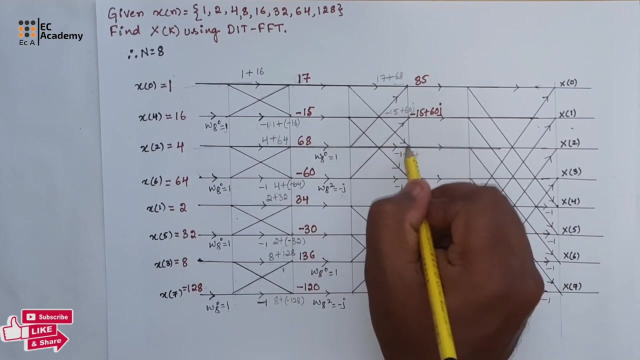 minus 15 plus 60 j To find output. at this point, let us take this input line, So, which is 68, into 1, into minus 1, it is minus 68, plus on this line it is 17.. So minus 68 plus. 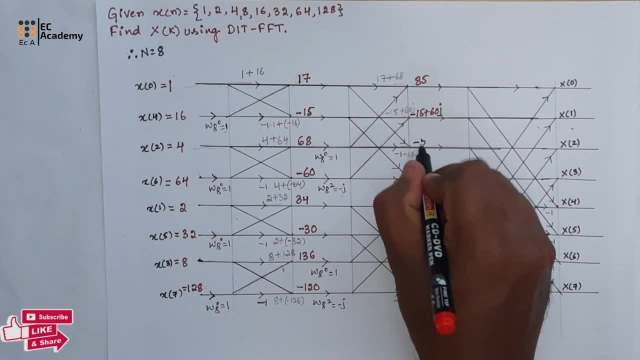 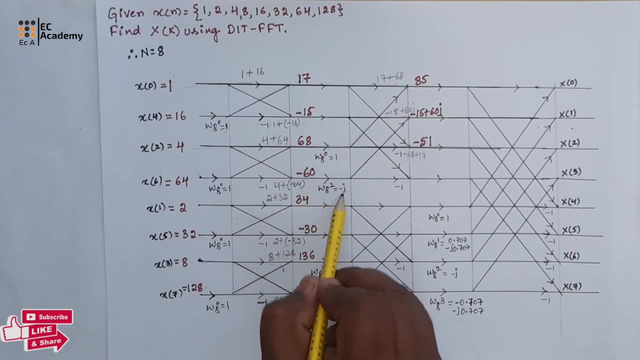 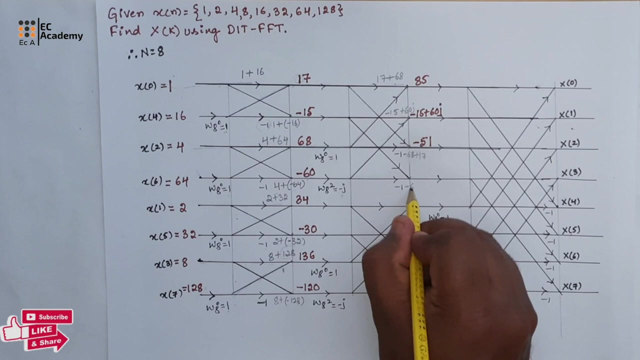 17. Output at this point is minus 51.. So output at this point again, it is 64 into 1, it is minus 60 into minus j. it is 60 j Here. it is minus 1.. So it will be minus 60 j On this. 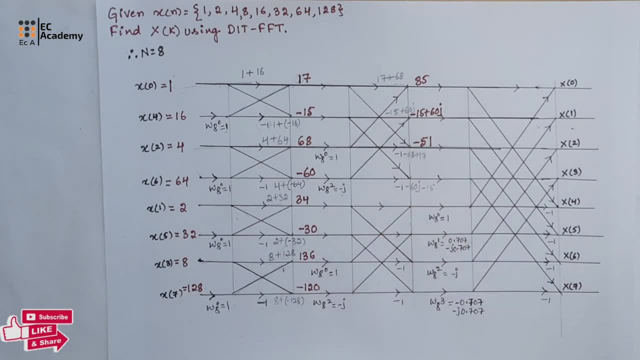 line it is minus 15.. So the output at this point will be minus 15 minus 60 j. Again, to find the output at this point, let us take the input- here it is 34- into minus 60 j. 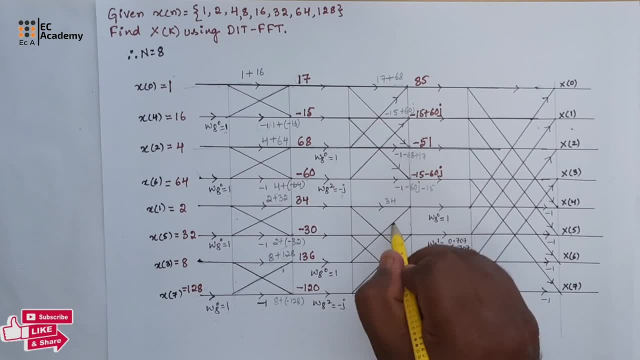 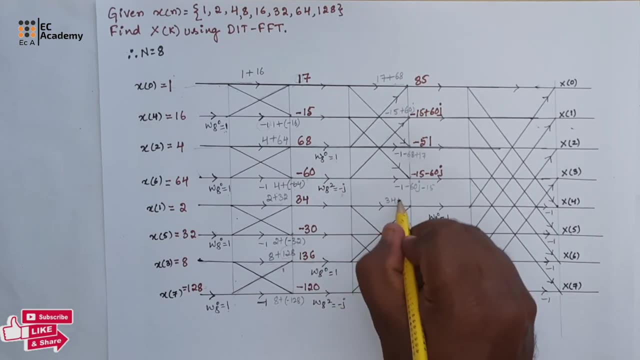 So the line which is joining this point is this one. So the input is 136 into 1 plus 136, it is 170.. So output at this point is 170.. In the same way, for this point it is: 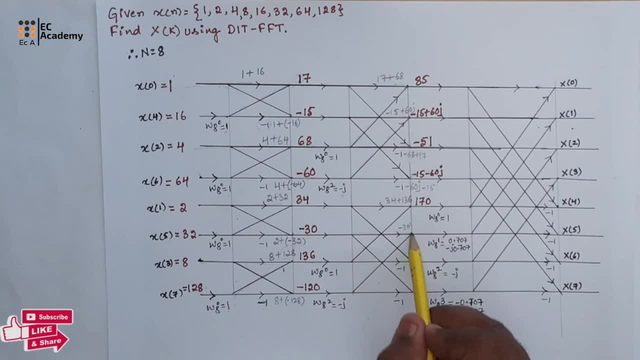 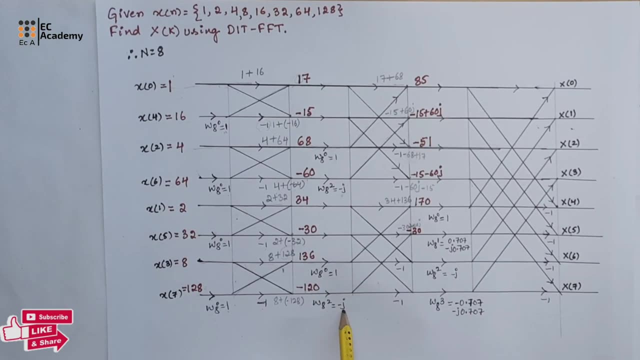 minus 30. So the line which is joining this point is this one. So input here is minus 120 into 1.. So the output at this point it is minus 60 into minus j. So it will be 120 j. So the. 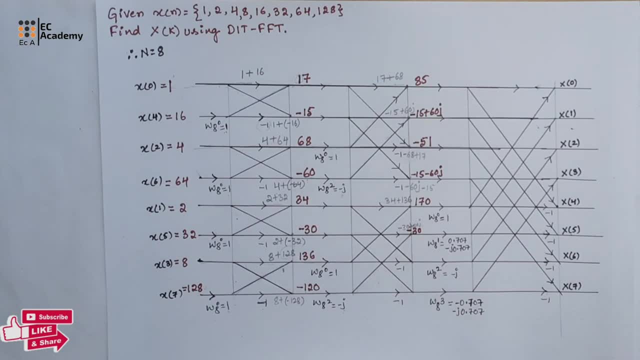 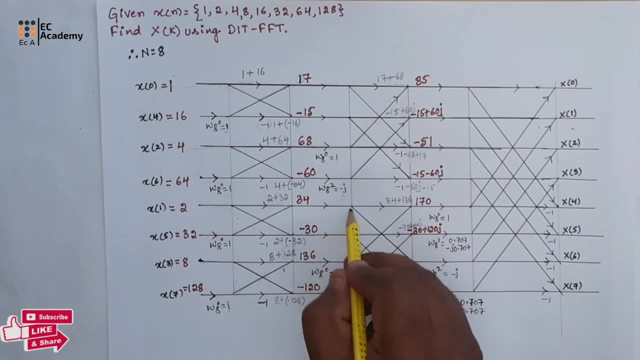 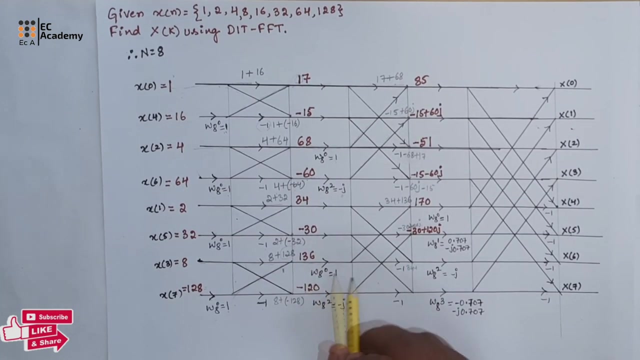 output. at this point it will be minus 30 plus 120 j. So it will be minus 30 plus 120 j. At this point it will be 34 plus 136 into 1, into minus 1.. So it is minus 136.. So minus. 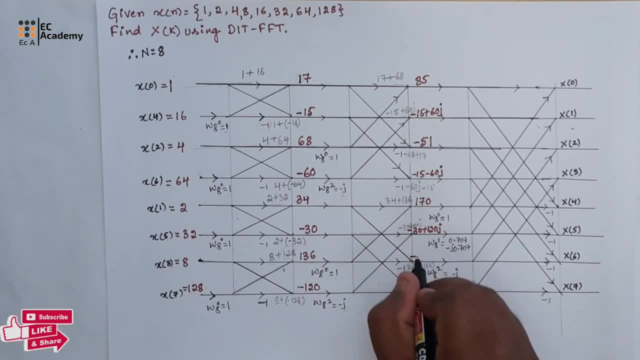 36 plus 34, it will be minus 102.. At this point output will be minus 30,. on this line it will be minus 120. minus j, it will be 120 j into minus 1, it will be minus 120 j. So the output. 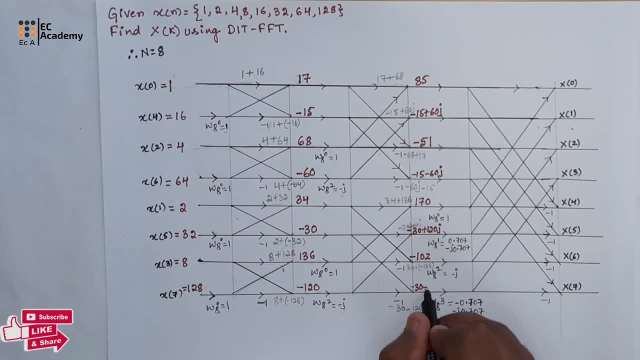 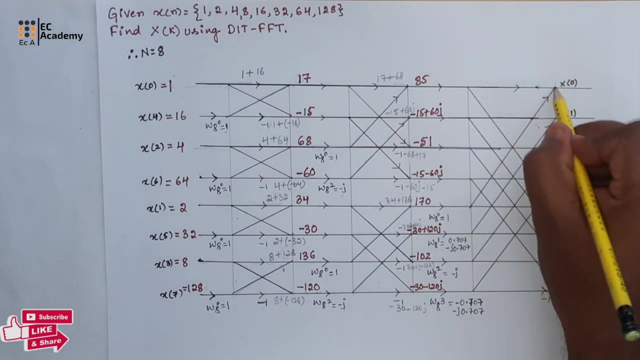 on this line will be minus 30, minus 120 j. Now this intermediate output will be the input to the next stage. Now we need to find x of 0, to find x of 0, at this point the input is 85 plus. so the line which is joining this point is this one. so the input here is 170. 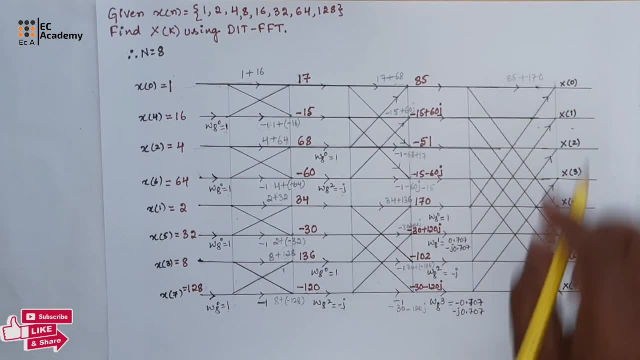 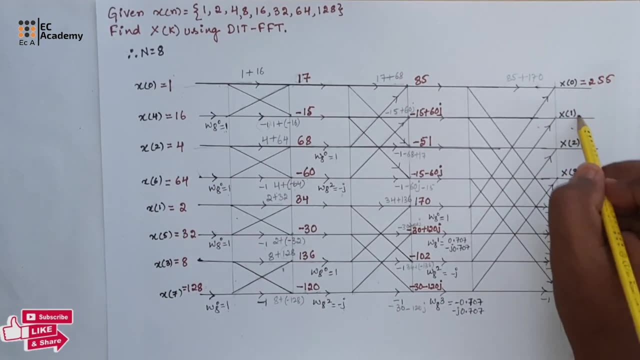 into 120.. So it is 170,. so the output at x of 0 it will be 255.. To find the output at x of 1, at this point it will be minus 15 plus 60 j plus. so input on this line is minus 30. 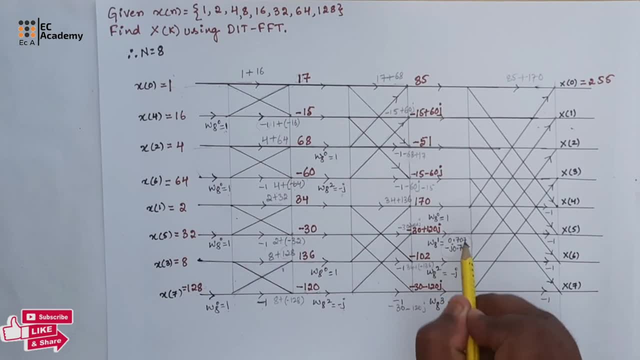 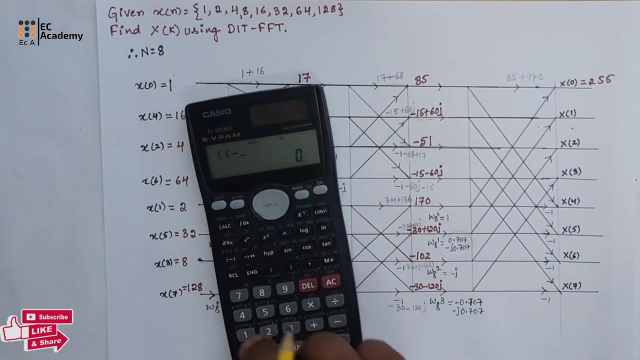 plus 120 j into 0.707 minus 0.707, so on this line, So you can use the calculator to calculate the output. So you can calculate this. so it is this value which is minus 15 plus 60 i plus. so on this, 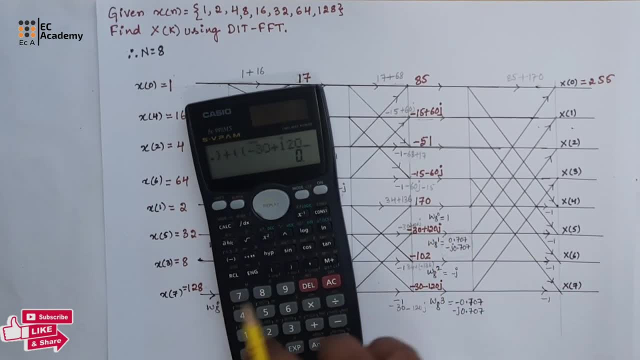 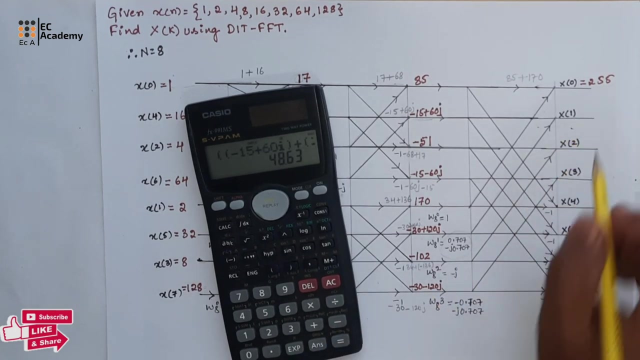 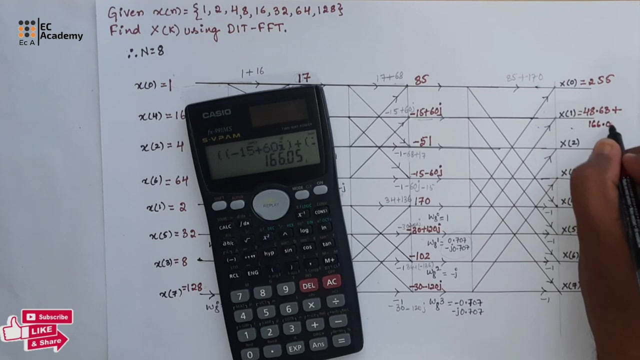 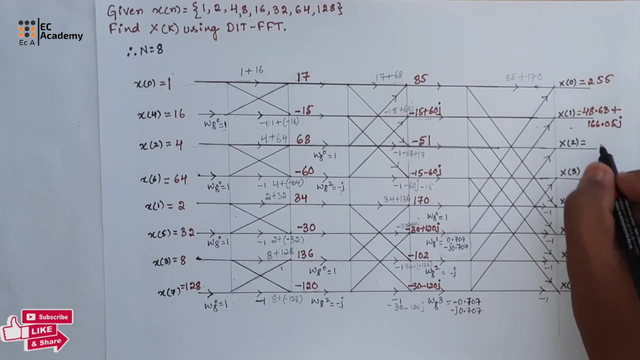 line, it is minus 30 plus 120 i into 0.707 minus j 0.707.. So the output is 48.63, shift equals plus 166.05 j. In the same way you can calculate for all these values: for x of 2, it is minus 51 plus j 1 naught 2. for x of 3, it will be. 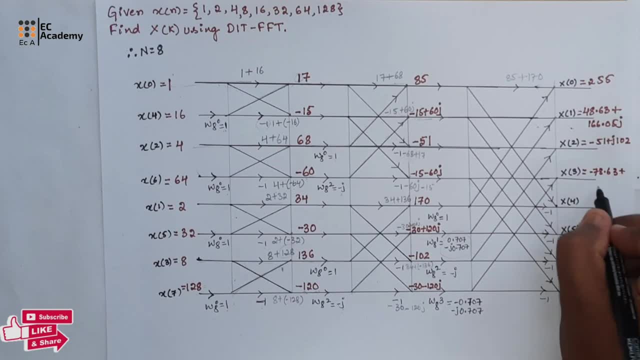 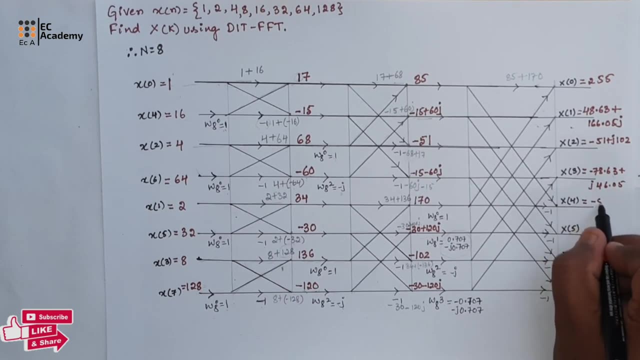 minus 78.63 plus j 46.05, for x4 it will be minus 85, for x5 it will be minus 78.63 minus j 46.05,, for x6 it is minus 51 minus j 102, and for x7 it is 48.63 minus j 166.05.. 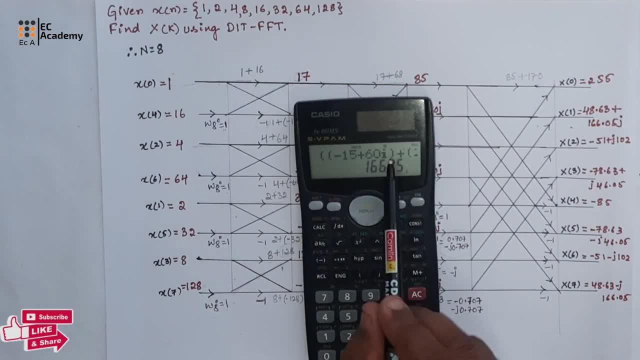 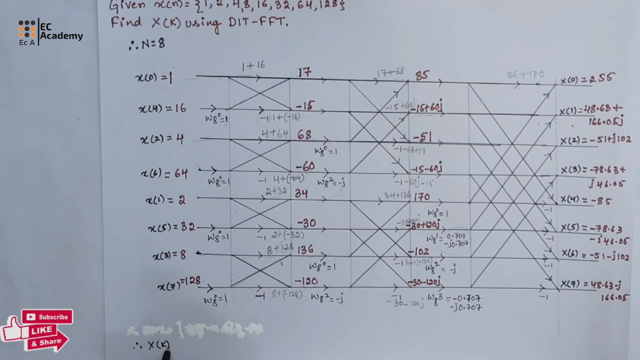 So while using the calculator, you need to keep the calculator in complex and radiance mode and perform the calculations. Therefore we are done. We can write: x of k is equal to 255, 48.63 plus j 166.05, minus 51 plus j 102, minus.